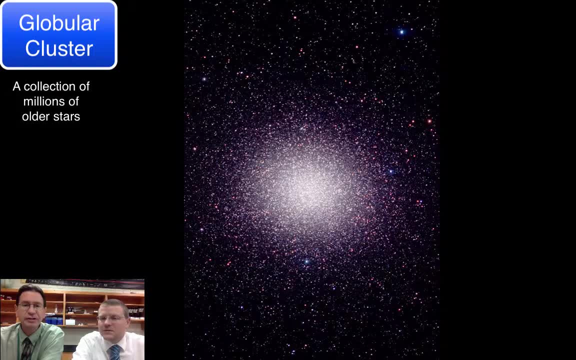 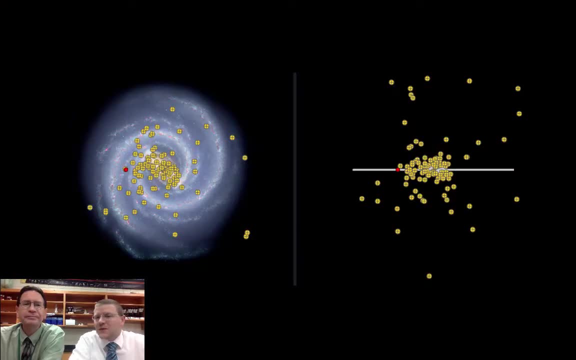 Now we can use these clusters to find distances, especially since these are located more towards the center. We can use them to locate the actual center of the galaxy, and this is what we see when we plot all those globular clusters. So the red dot is the Sun and all the orange dots are the globular clusters. 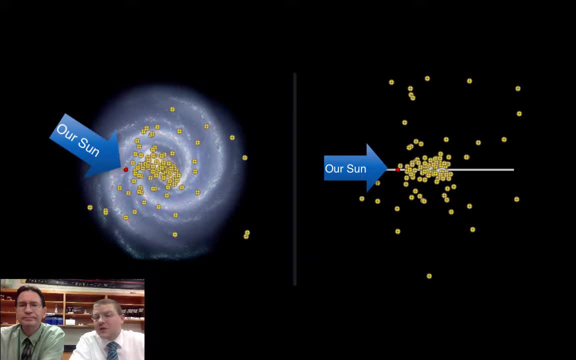 If the globular clusters are hanging out around the center of our galaxy, we see most of them skewed off to the left or right. We see them not surrounding us, which tells us that we're not in the center of our own galaxy. So now we know our 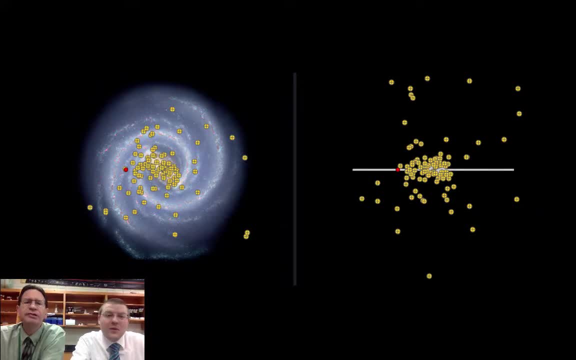 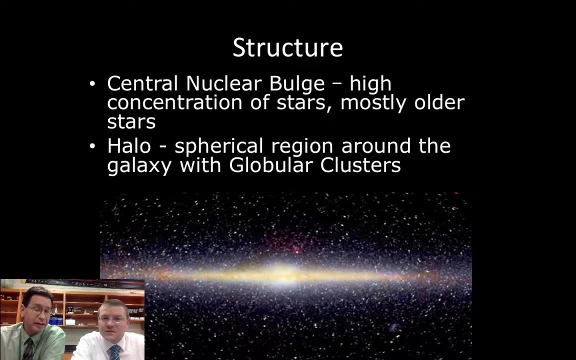 location in the galaxy. The next thing is we want to talk about the different parts of the galaxy. Yeah, so you can look here and you can see that the galaxies, especially our type of galaxy, has a definite shape to it. It has a bulge in the center called the central bulge. There's a lot of stars there, and they're mostly the oldest stars. 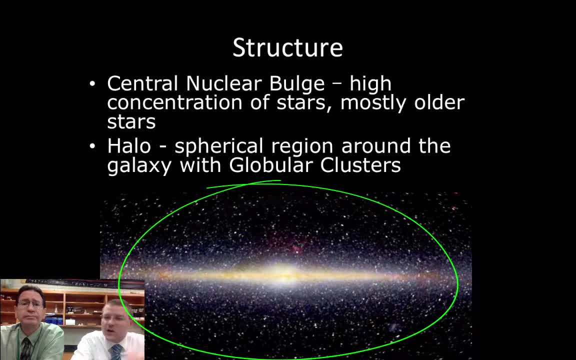 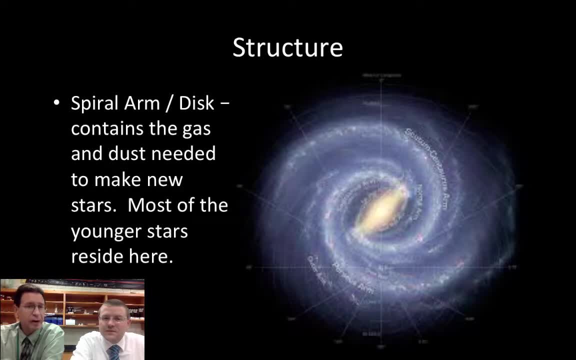 Around the galaxies. we call that spherical region, the halo, where all those globular clusters hang out. What we view as the Milky Way is part of the spiral arms. It's part of the disk of the galaxy. A lot of galaxies are in the center of the galaxy. 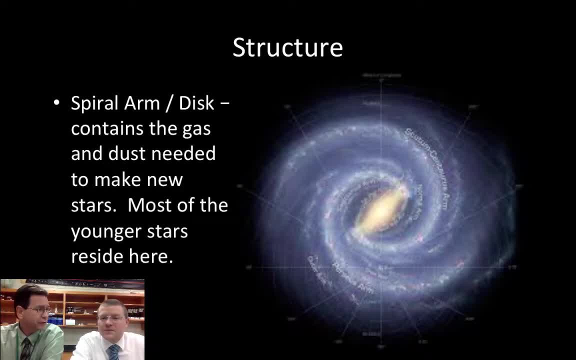 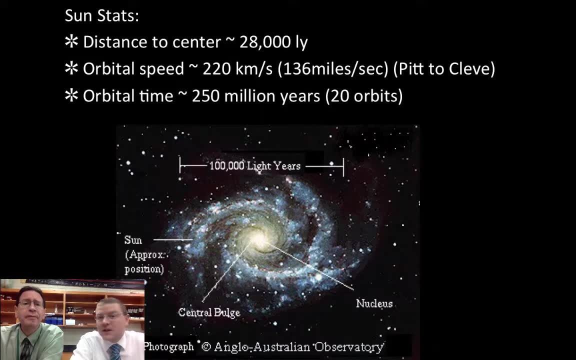 Gas and dust is needed to make this, and most of the younger stars are in this section. And again, if you want to pinpoint our location, you are right there. Some of the statistics about where our Sun actually is in the Milky Way galaxy. The galaxy is huge. It's a hundred thousand light-years across. 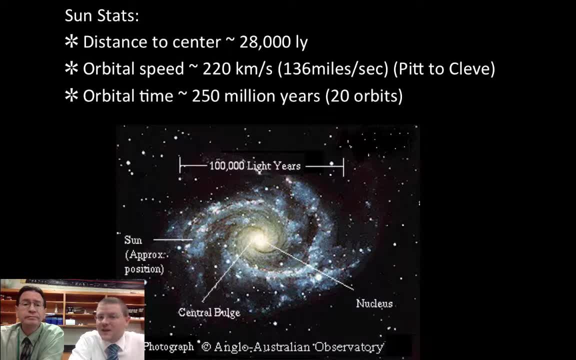 The distance to the center is about twenty eight thousand light-years. The Sun is moving very, very quickly as it orbits the galaxy. so it's moving around that central bulge And based on our speed, we know that it takes around two hundred fifty million years for us to make one orbit. 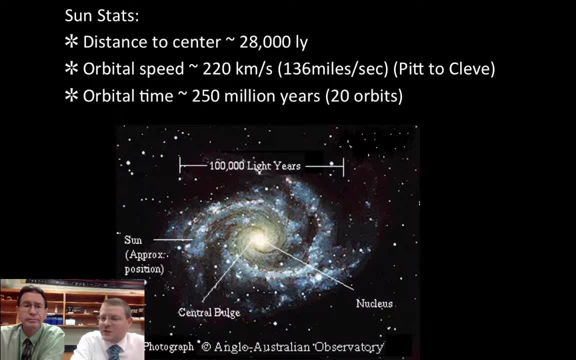 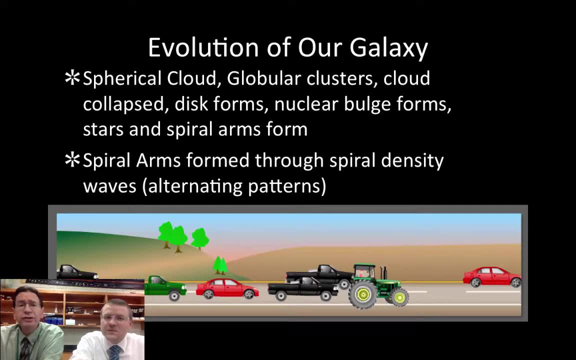 That's a long time, Which means in the Sun's lifetime it's already made about twenty orbits around the galaxy. The galaxy gets its shape basically by gravity, So there are clouds of gas, globular clusters, there are all these things that make up the galaxy. 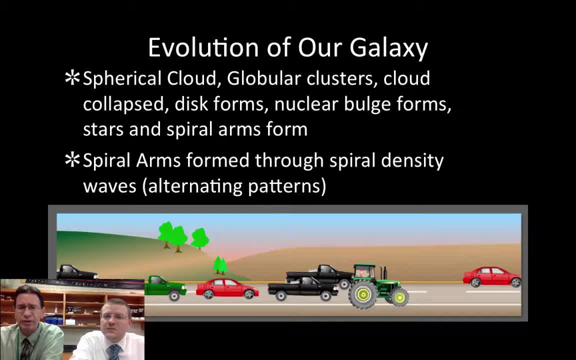 And gravity is sort of creating a situation where it forms a spiral And gravity is sort of creating a situation where it forms a spiral And gravity is sort of creating a situation where it forms a spiral And gravity is sort of creating a situation where it forms the arms. 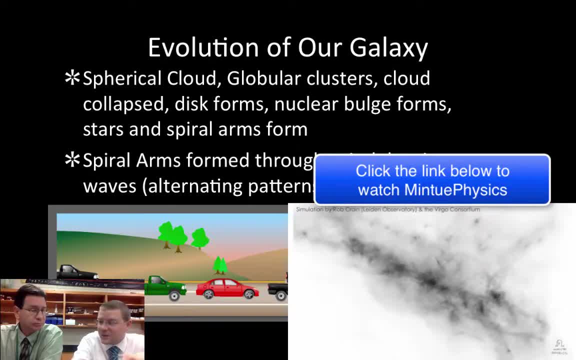 You've got the spherical cloud of gas and dust collapsing. First stars are being born. Those are the ones in the globular clusters. The cloud collapses into the flat disc. The flat disc rotates. The nuclear bulge has some of the older stars in a high concentration, the stars in the middle. 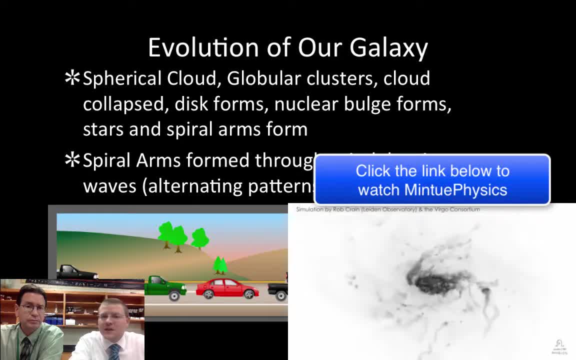 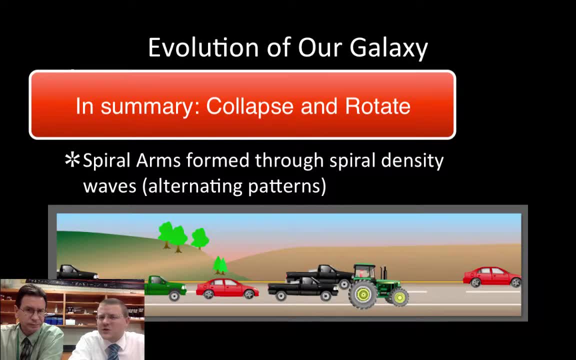 And then the spiral arms spin out, giving us the shape that we have. But why do we have definite, defined arms? That's one thing that astronomers are trying to understand, trying to wander. One of the ideas is something called a spiral density wave. 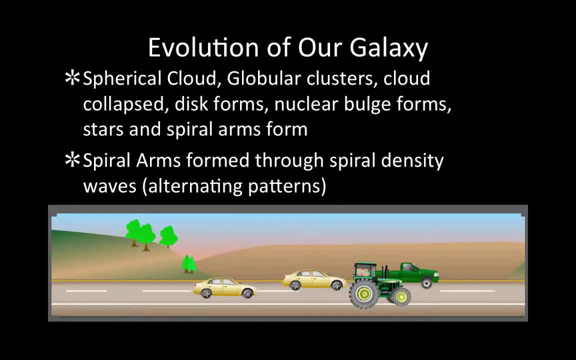 where the gravitational fields of these stars, the arms, all of this material is sort of separating. It's kind of like traffic separating at traffic lights. The gravity causes a gap between sections of the disk and it makes the arms. So you got slower moving material like this tractor right here and you can get stars. 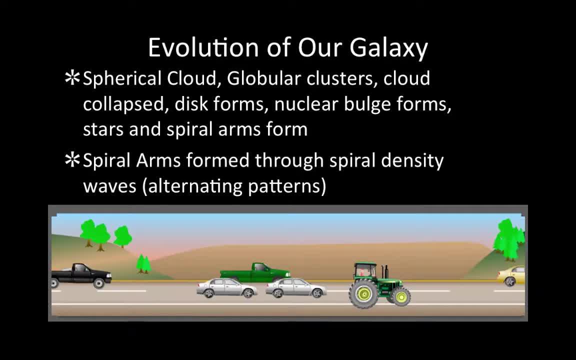 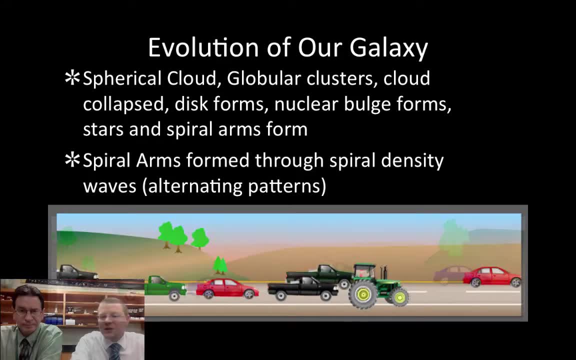 and gas to clump up behind it. So we have those different regions, like in a traffic jam. That's why we're getting the densely packed spiral arms, the spiral density wave. To sum up here, you can see the halo is around the galaxy. That's where 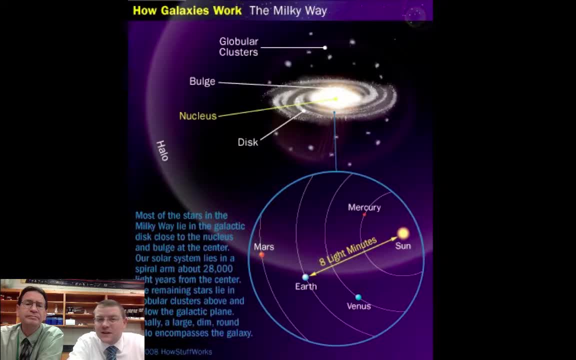 the globular clusters hang out. Then you've got the disk of the galaxy where our Sun is located and a lot of the gas and dust to make younger stars. In the center we've got the bulge of the galaxy where, we said, a lot of older stars are. 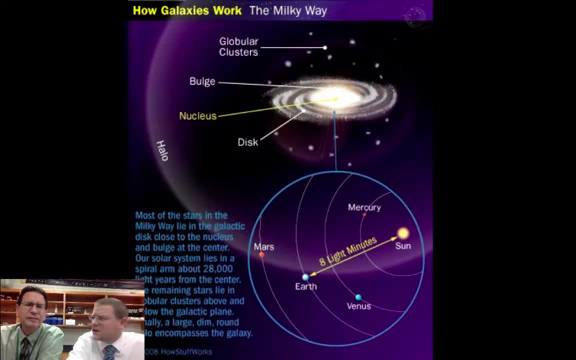 but then there's that word nuclear. What's in the nucleus, or the center of our galaxy? Another question might be: what's holding this all together? because I think what's in the nucleus is something that's doing that. So when astronomers peer into the 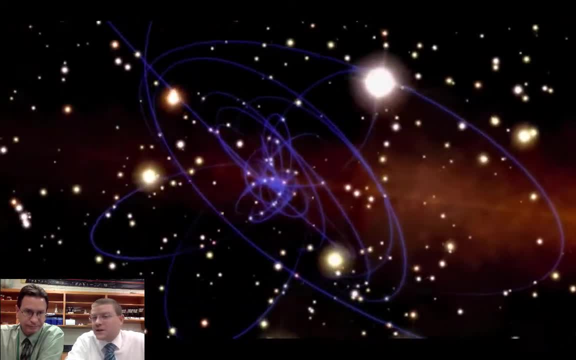 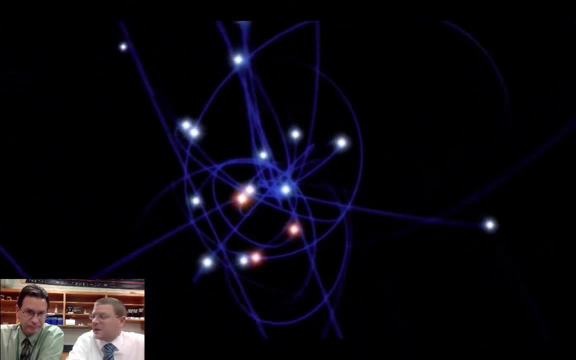 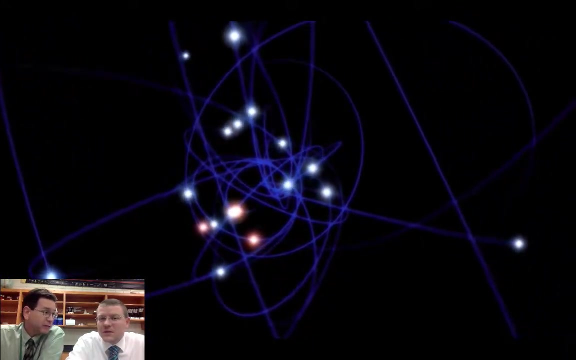 center of the galaxy, which is centered around the constellation Sagittarius. they focused on a bunch of stars kind of orbiting something. Yeah, it almost looks like water flowing down a drain. They're going around and round in circles pretty fast for stellar matter. 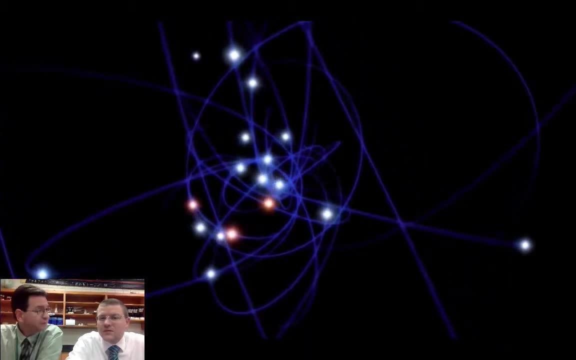 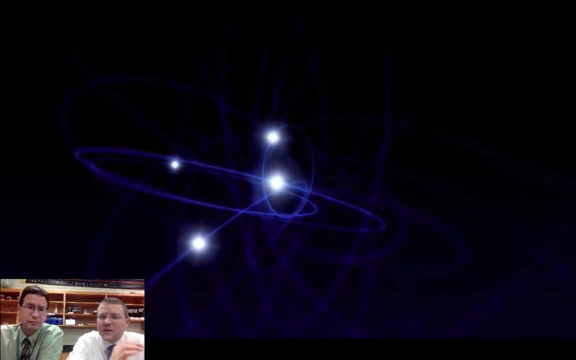 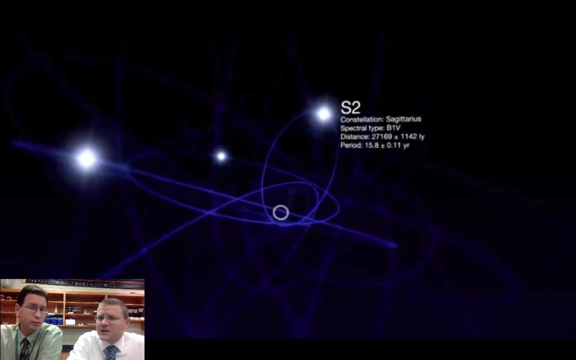 They like solar motion, so there must be something there that's causing them to spin. So, doing some calculations and mathematics to figure out what the mass of that central body must be, the mass of the central body ended up being around four million times the mass of the Sun. That's got to be something that's.